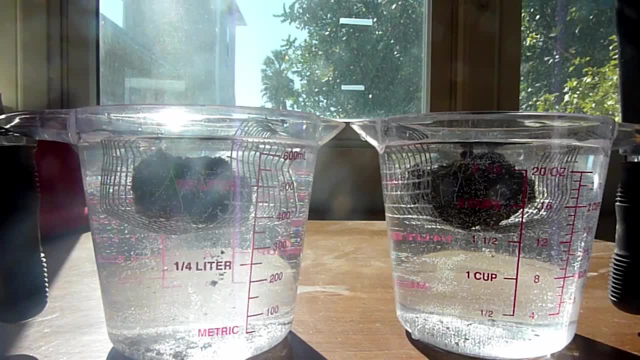 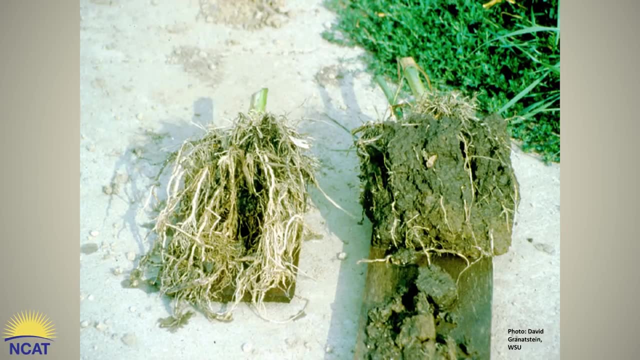 glues, along with fungal mycelia and plant roots, hold the soil together. This picture shows the difference between a healthy and a poorly managed soil. David Granatstein, a sustainable ag specialist at Washington State, dug up two corn plants in fields with the same soil type, but which? 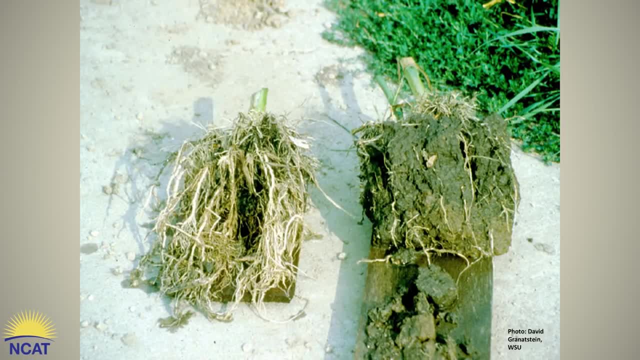 were managed differently. He applied water from a garden hose to both root balls. One field used a lot of chemical fertilizers and pesticides, no cover crops, a lot of heavy machinery and a poor crop rotation. The other field was not organic but used manures, cover crops and tried to minimize tillage and heavy machinery use. 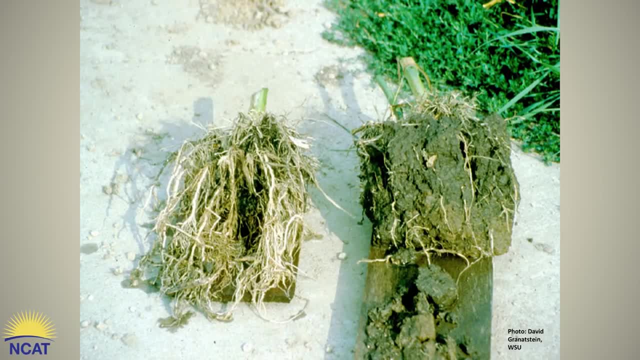 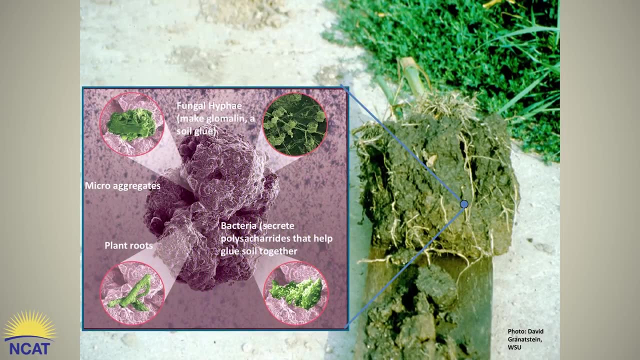 David noted that the soil on the root ball on the left immediately washed away and nearly all the soil was gone after 30 seconds. The soil with the root ball on the right resisted washing away due to the presence of soil glues which were present due to the farmer providing food in the 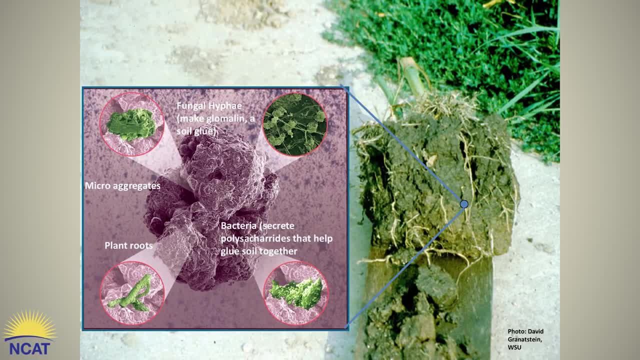 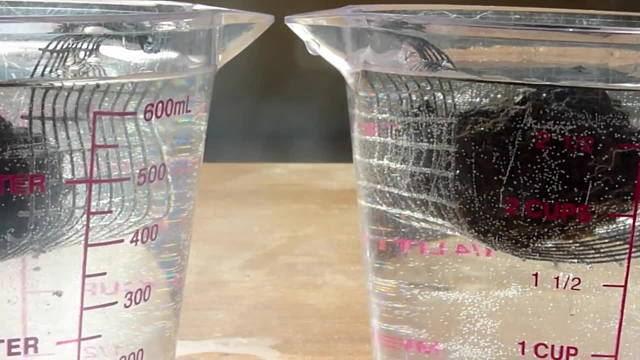 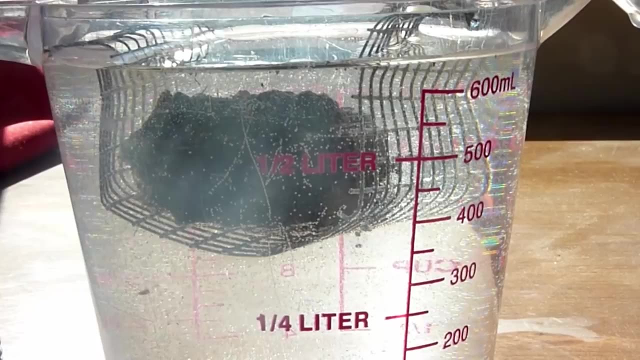 form of manures and cover crops to the soil ecology. The situation shown here is similar to the corn root ball example. The soil clumps are the same soil type and were taken literally feet from each other from two adjacent orchards which are managed quite differently. The soil on 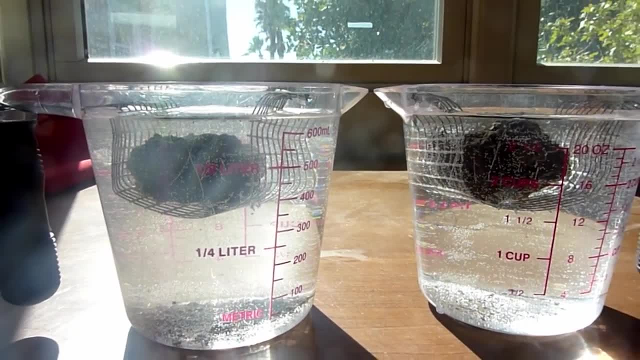 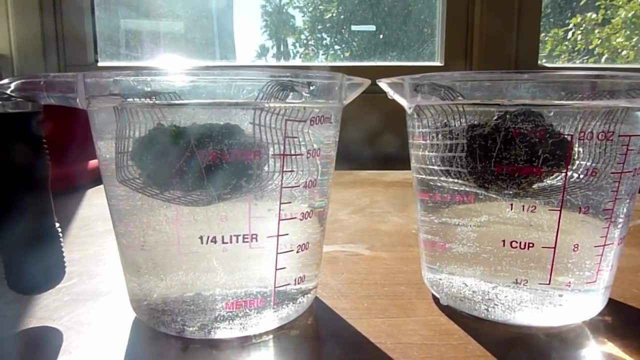 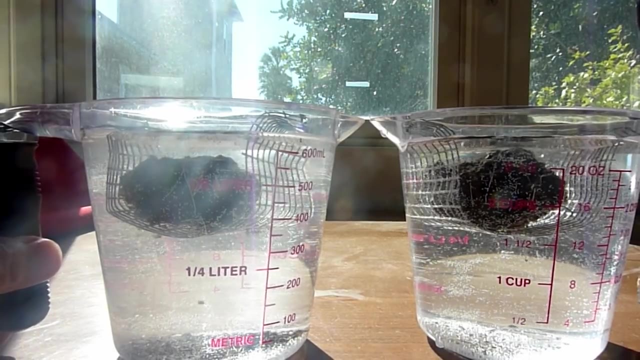 the left is from an orchard where the alleys were kept clean of any vegetation through the use of herbicides, So very little organic matter is returned to the soil and the soil is starved of organic matter. The soil on the right is taken from an orchard that has cover crops planted every year in the 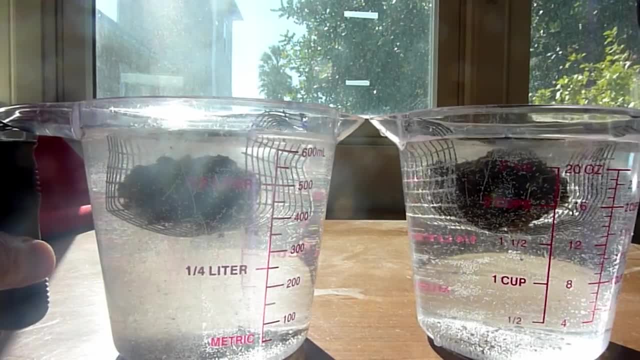 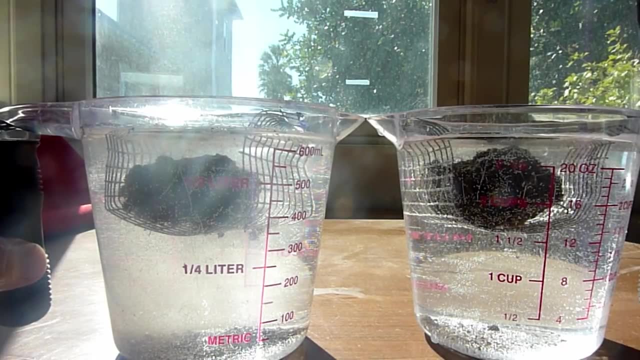 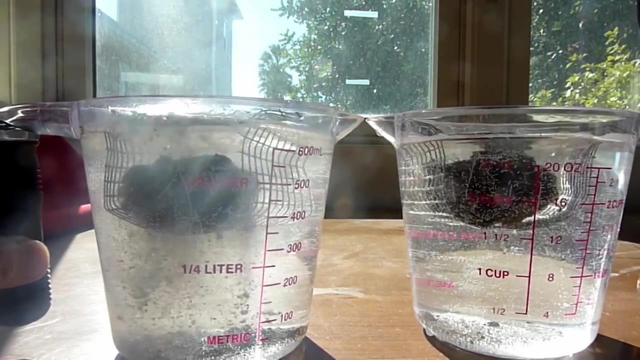 alleys and has also had animals grazing in the alleys. The soil resists disintegration when exposed to water. As you can see, even though the healthy soil on the right does disintegrate a bit, the water remains clear because the pieces that fall off are micro aggregates. so most of the clay particles remain aggregated. So back to why having stable aggregates are important. First, healthy soils which are well aggregated resist wind and water erosion by maintaining their structure. Heavier aggregates are more likely to stay put compared to particles of silt, sand and clay If the soil disintegrates. 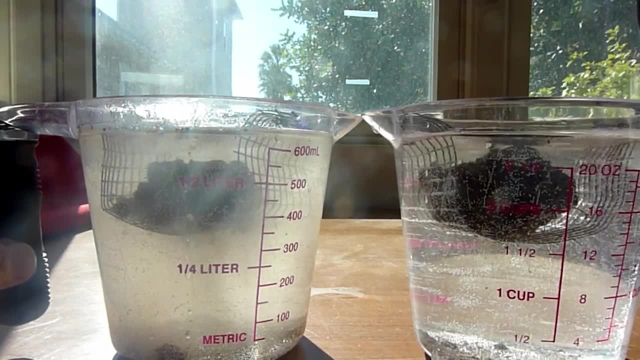 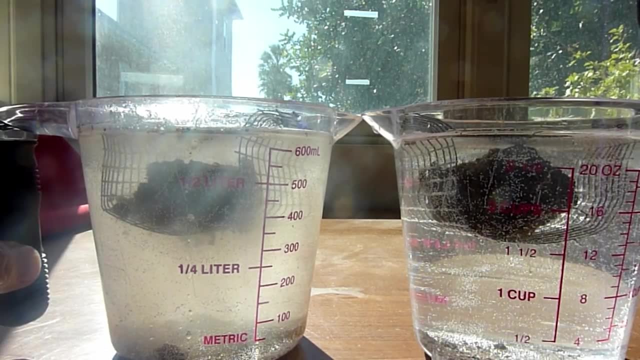 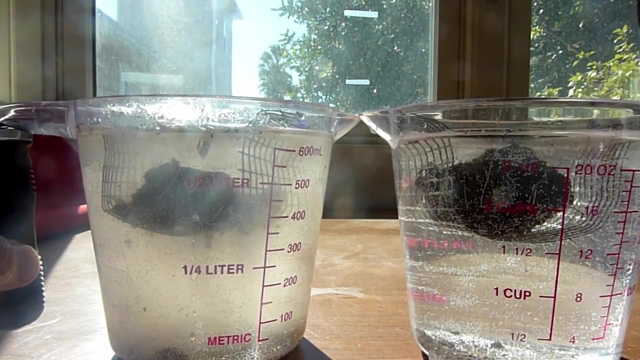 as the soil on the left is doing, the clay particles will rise to the surface and form a seal, after which very little rainfall or irrigation water will penetrate the surface. The roots and, ultimately, the water table are starved of water. In addition, the clay seal dramatically reduces